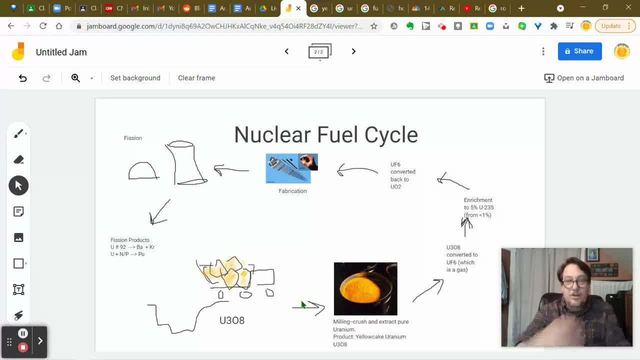 or electrical processes into what's called yellow cake uranium, which is this stuff here, And it is also U-308, but it is now not just little dots here and there in the rock, It is a more pure form Still not usable in a nuclear power. 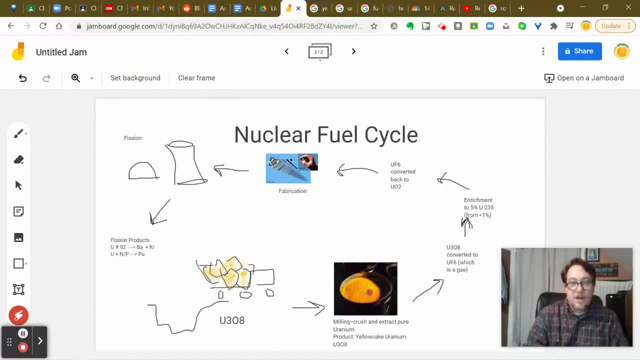 plant, but now, for a different reason, sort of. It's more concentrated into a purified form, but it still isn't concentrated enough as far as the isotopes that will fission. Remember that uranium-235,, which will will fission, is less than 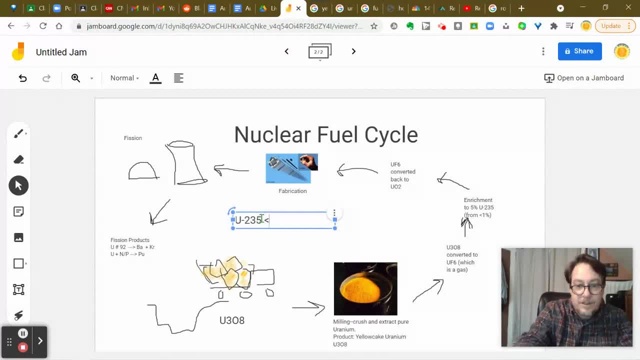 Whoa, come on now- is less than 1% of a sample, whereas you need it to be- Oh right, You need it to be 5% for power, And the rest- Almost all of the rest- is uranium-238.. 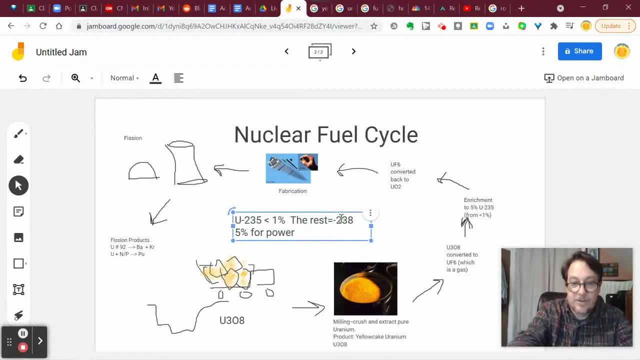 Now, of course, I talked about this in the thing last week, so I'm not going to go through the whole process, But just as a reminder, that's why this next step happens, which is the enrichment. That's what you see over here. 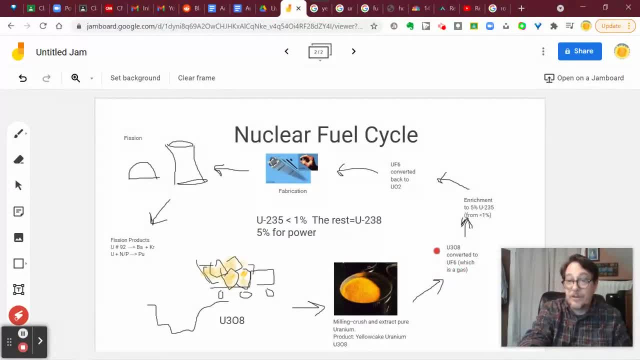 There's two steps to enriching. The first thing is that you take the, the? u, the uranium oxide, the uranium oxide, and you convert it into uranium hexafluoride only because it's a gas. You need it to be in gaseous form to do the gaseous diffusion process. 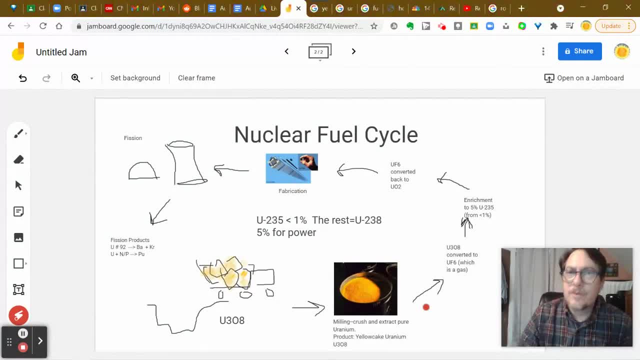 Interestingly, I was just in Paducah, Kentucky, which is where America's gaseous diffusion plant is, or was one of the the main ones. I'll have more to say about that later in the course, But anyway, they turn it into a gas and they put it through the centrifuges and they enrich it. 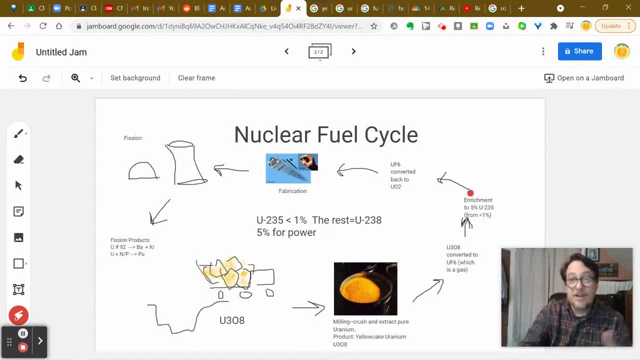 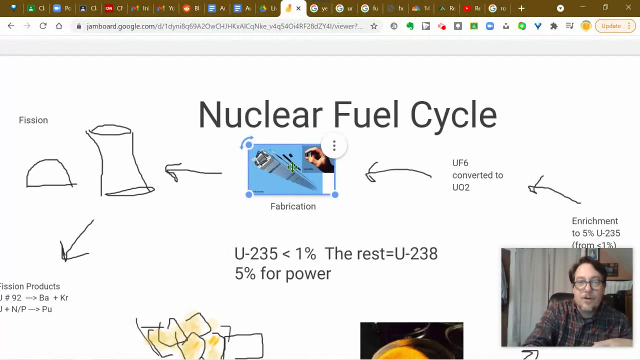 At which point they have enriched UF6, which then has to get converted to uranium oxide, UO2.. So not Bak2.. Let me correct that Is to be converted to uranium oxide, And then it's turned into fuel pellets. Let me just grow this real quick so you can see what I'm talking about. 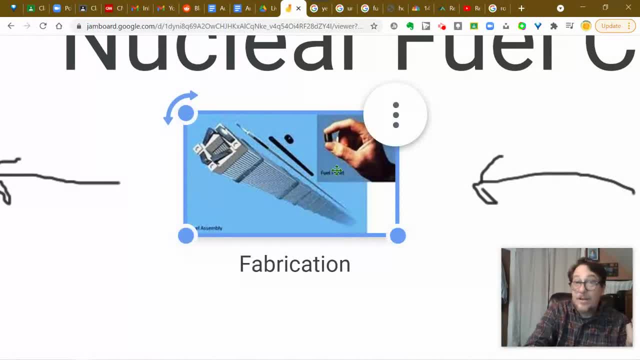 That's a uranium fuel pellet there, held between the fingers- fingers. Oddly enough, that's not an unsafe thing to do, Don't? uh, it's okay, But that is a. it's not pure uranium, uranium metal. It's a pellet that's uh composed of a ceramic matrix with the 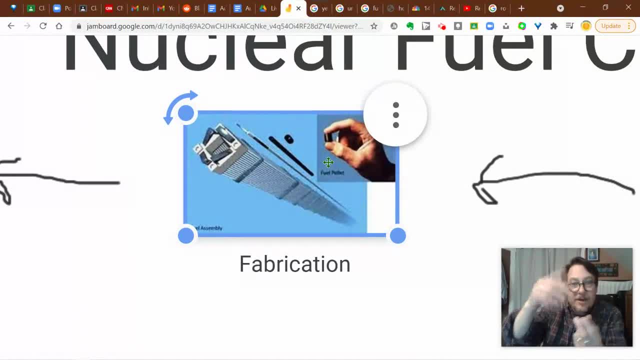 uh, uranium oxide or U2, yeah, the uranium oxide embedded in it in a matrix, And then you can see that that's uh may fabricated into a larger rod, into a a longer uh rod, and then the actual 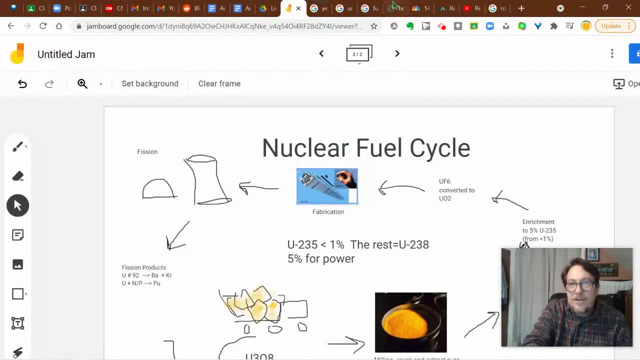 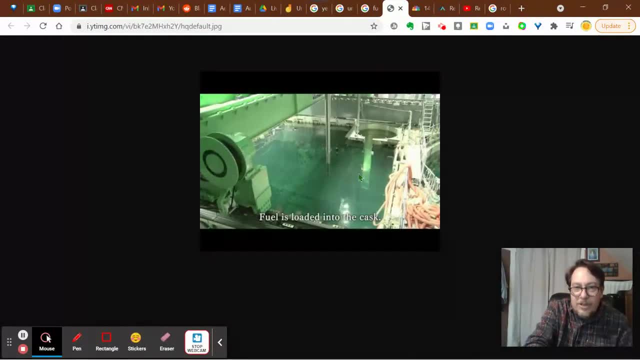 fuel rod assembly, of which, let me see here I have a picture. Yeah, here's, uh, this is one of those assemblies here being loaded into a fuel pool, and you can just make out the tops of all of these. So all those little squares, like you see. 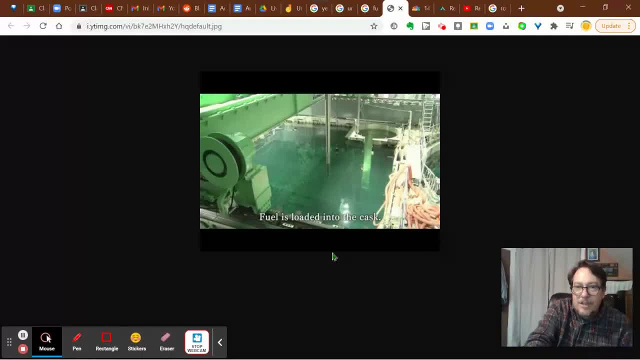 there. that's basically what you're seeing: All those little tops lined up, uh, and this thing is being lowered down into there by machine, Although with the 20 or whatever feet of water it is here. that blocks, that effectively blocks even that massive amount of radiation release that's in. 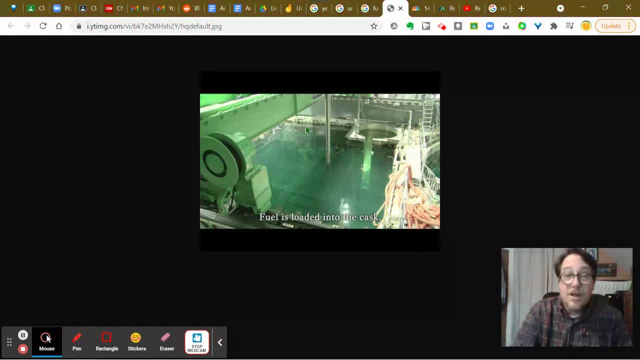 there, And you can't even imagine how much radiation is in there. but the the water blocked it, And so you could, if you were so inclined, walk along the uh, the edge of the pool. no, running in the pool, uh and uh. 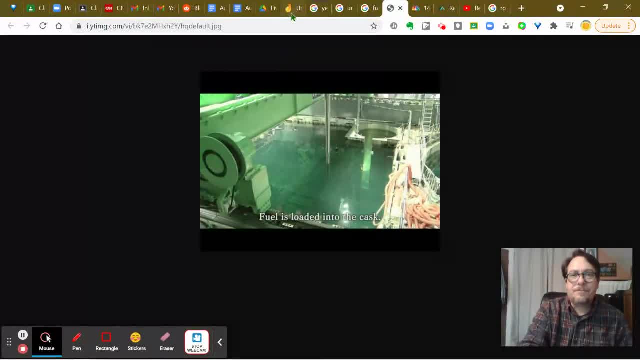 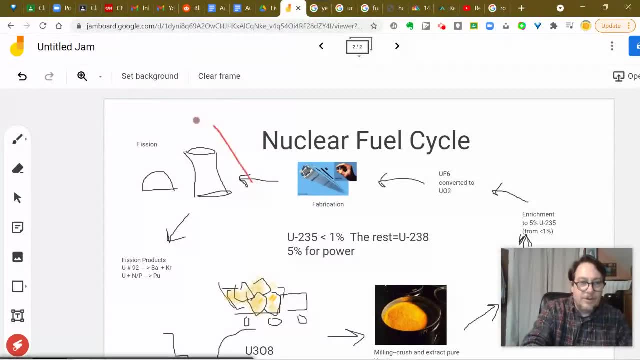 there, you have it. So okay, But anyway, you wouldn't be harmed, All right, And so that's the fabrication of the fuel. And to get to the last point, we, you, you, learned about the fission and the thing I made before, And so the fuel is used in the nuclear reactor. I think a? um, I know that. 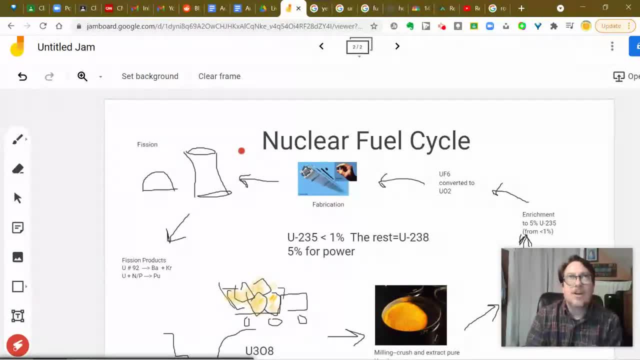 the fuel has changed every 18 months and every uh, I think a particular pellet will go through three cycles. So they change out a third of it every uh 18 months, And so 36,, 40,, 54,, 54 months, Uh, so that about four and a half years uh, a fuel pellet will be. 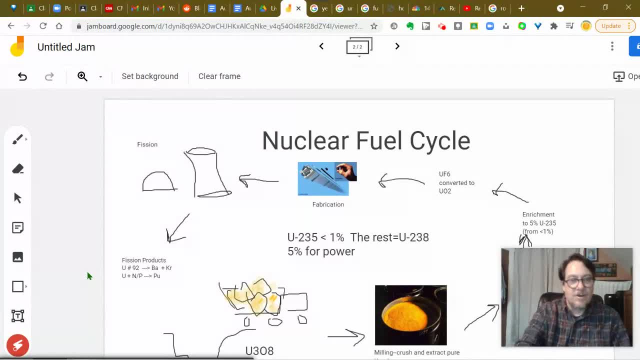 in there And I could be getting that wrong. but and then what you're left with are the fission products, And we're not going to have that much time. If we were doing a five day a week class, we'd spend three, two or three days on just the fission products and talking about them, But just 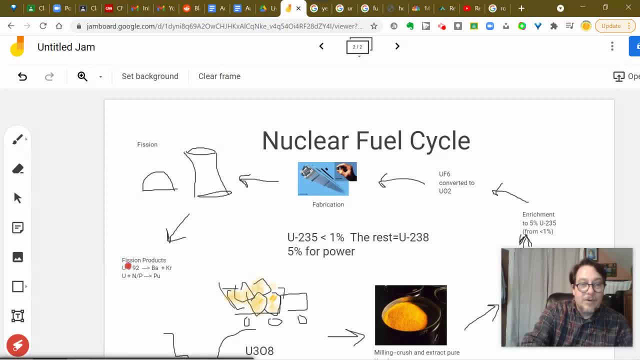 to give you a brief look. the idea is that if you're, uh, you're, using baryonium as the fission, um, you become a piece of paper and you break everything together And uh, so, if you think about it, if, uh, what's baryon? number 56, 56 of those protons. 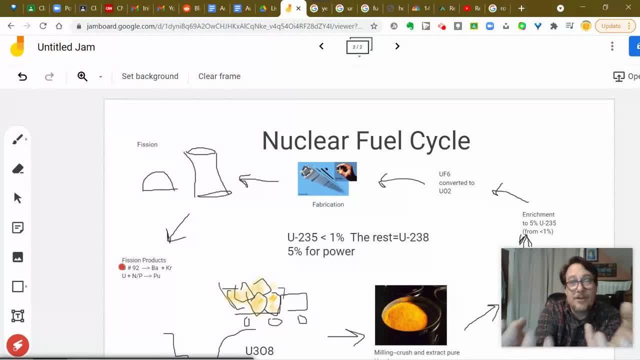 are in one piece and that leaves 36 protons in the other piece. that's baryon and krypton. Those aren't the only pieces that can be created. Uh, strontium and xenon. uh, is another another thing that could happen. 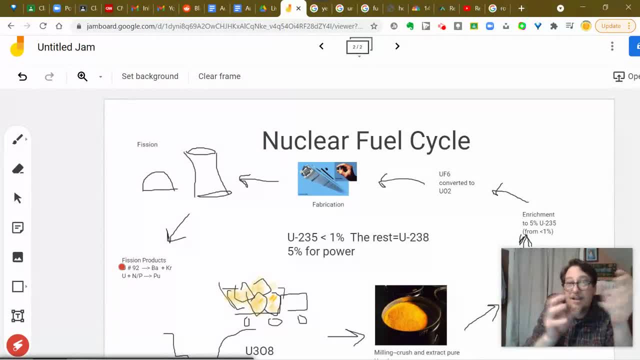 a lot of. there's a lot of different combinations, because the egg doesn't always crack exactly the same way, but it does crack, it does, uh. and another thing that can happen is that, um, there's a lot of intermediates in this and this is some nuclear chemistry here and i'm not going to get it all. 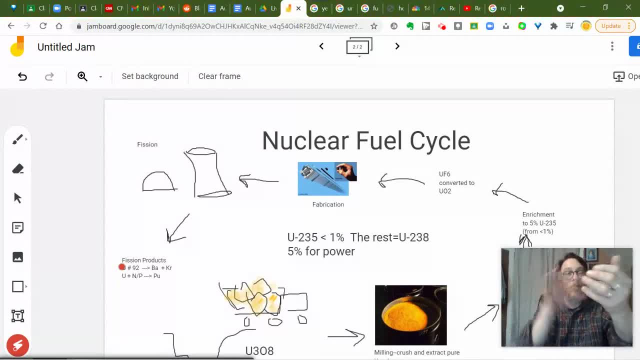 out for you. but you can end up with something bigger: the, the nucleus absorbing particles, and in that messy fission process and uh, one of the unfissioned uranium takes on two more protons and becomes plutonium, which is number 94.. plutonium is an? uh, an artificial element that's only created by 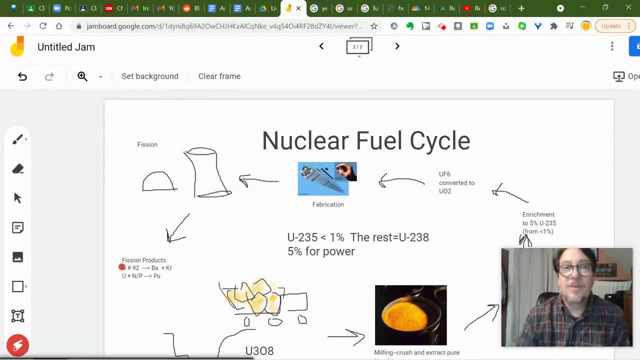 this, but it's also bad guys. uh, plutonium is a is the most poisonous substance, ounce for ounce, in all of the world as far as we know, because a lot of reasons, but one of them is that plutonium is a perfect minimum of plutonium and plutonium is a perfect minimum of plutonium and plutonium is a. 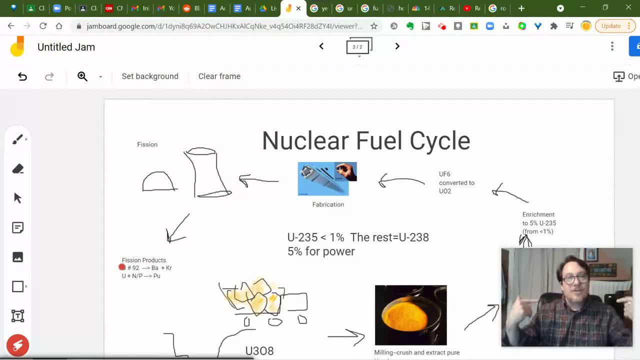 mimic for calcium, and so if you get plutonium in your system, the, if it's going around your bloodstream and it gets to, let's say it's going through the canicula of your bones, uh, and it needs some calcium. it's like i'm calcium and your body's like: cool, here's some calcium. and now 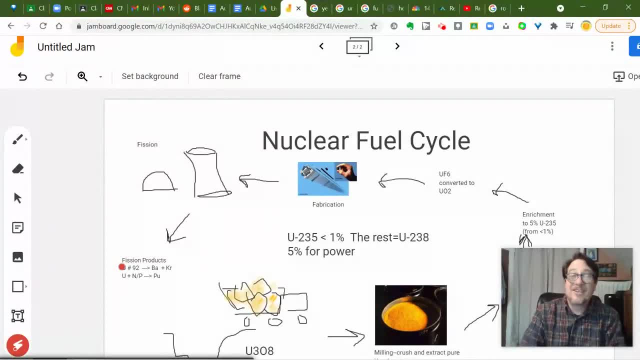 you have plutonium in your bones. i think that's all you have to say to know that that's not good. and so, anyway, this is why these nuclear- well it is, it is a nuclear waste. nuclear wastes are clearly dangerous, and they are. for a long time. we haven't talked about half-lives again. another. 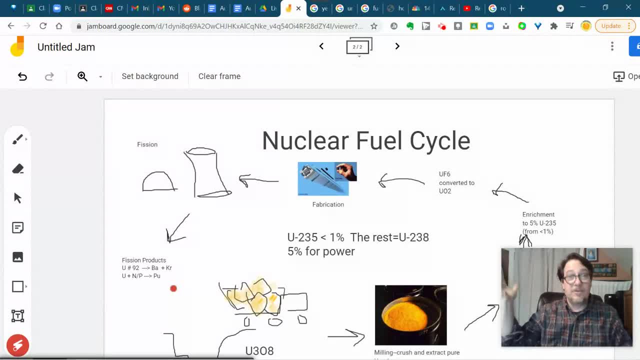 topic we're not going to get to talk too much about, but a half-life is the amount of time it takes for a radioactive element for half of it to decay into something else that's more stable, and so the half-life for half of any sample of plutonium is, i think, 20 000 years, and you have to. 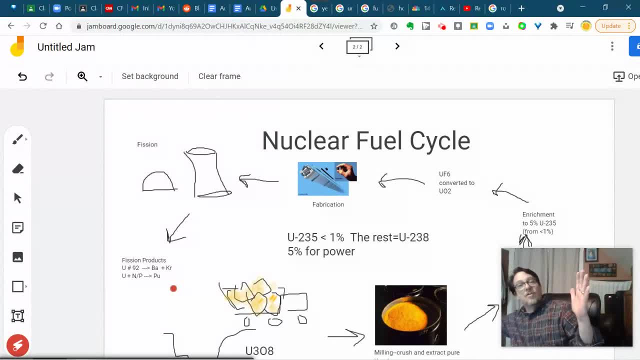 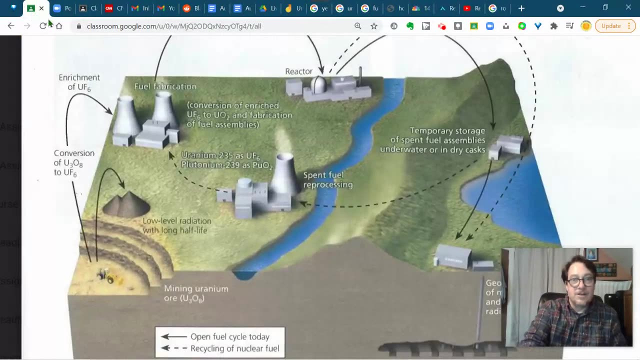 go 10 half-lives before it's considered gone on. some even say 20.. that's what? 400 000 years, right, two to four hundred thousand years. uh, so the wastes are a thing, and actually let me go to your reading here, if i still have it up. 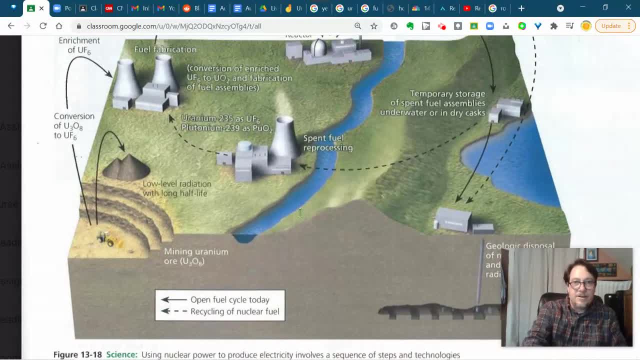 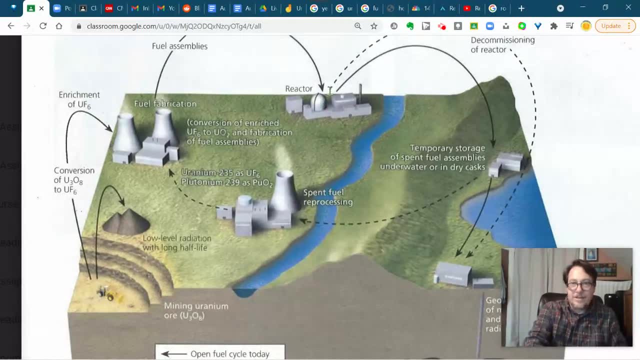 that's right. here's the whole thing right. and as you go through the part, the fuel fabrication and the fissioning in the reactor, um, everything's stored temporarily um on site, either underwater in a fuel pool or in dried casks. uh, there is no intermediate place. they show it going somewhere else. actually, it's all still stored on site. 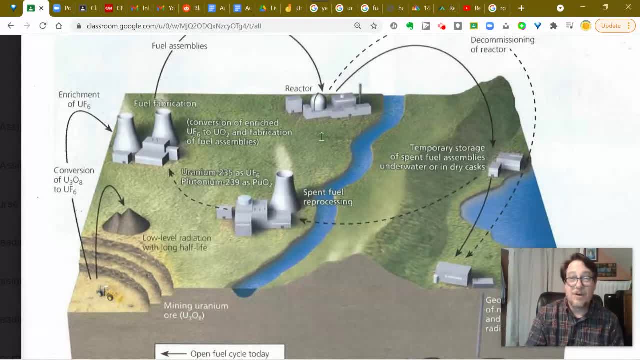 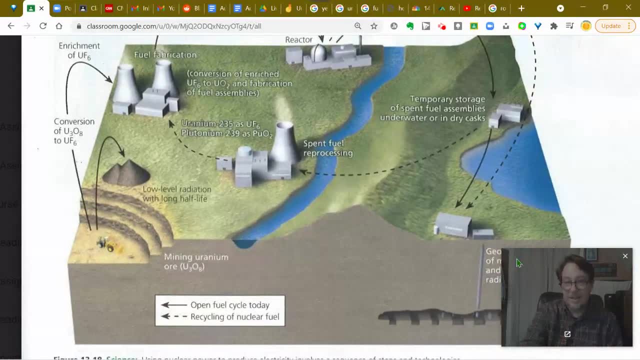 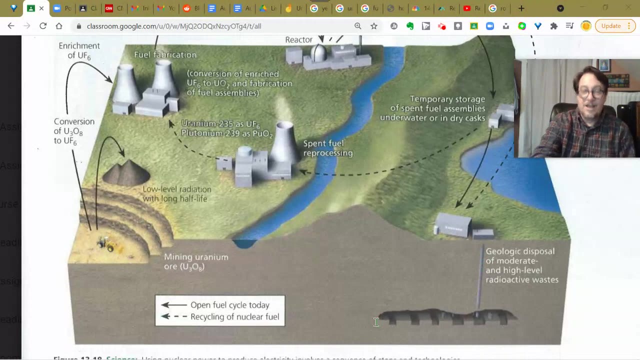 every. there's 103 nuclear reactors in the united states for power and they all, 103 of them- have their waste on site. there is no final place. there was an idea of creating what was called final deposition- geologic disposal of moderate and high level waste, and underground system that was supposed to be created where you could park that stuff and it. 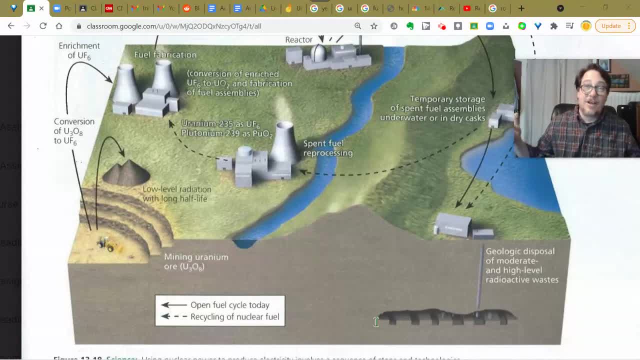 was geologically inactive- meaning earthquakes, hydrologically inactive, meaning water, and that it would stay that way for the requisite. you know it's actually much longer than the 200 000 years, because there's some things that are dangerous for a longer time. but even then people were skeptical. 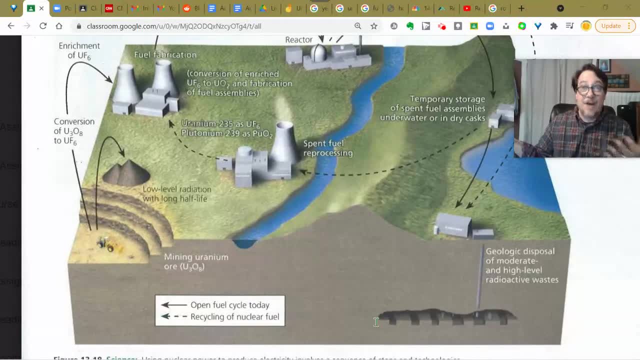 nobody wanted it in their state, and even nevada, which is you know was picked for it was, uh, fought so hard against it that the thing's been shelved so out of the purport to today. that one is the most shelf i've ever made. 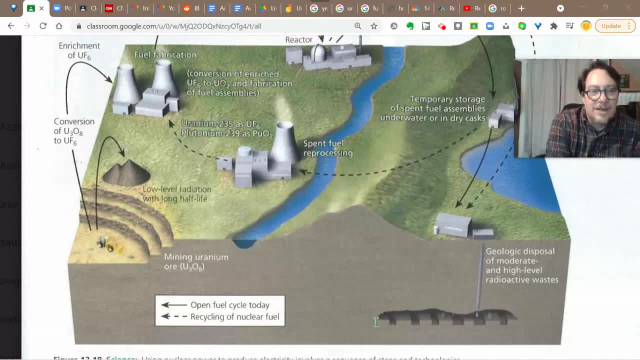 there's a lot of other issues to talk about with it, but i'm not going to get into that with you right now, because that's just another part of the cycle. another thing to mention is that there is, uh, this thing, this other little arrow that goes off here, which is called spent fuel reprocessing. 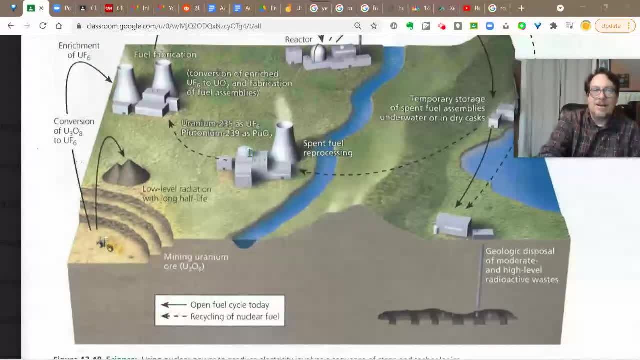 and the plutonium and other things. first of all, most of the uranium isn't used in that fuel pellet when it isn't fissioned, because what what happens is as it's fissioned. I don't know why I'm going like this, but on the outside, 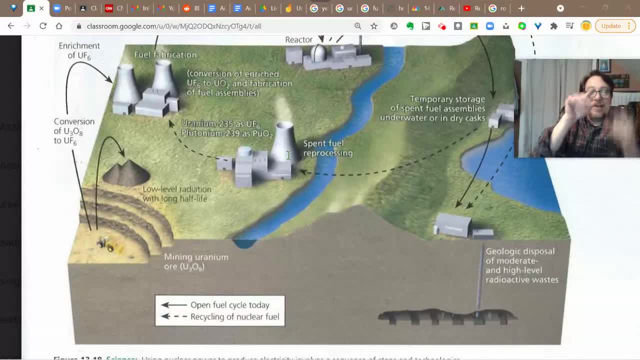 is where the reaction happens, And as they react, they create a coating that's impenetrable to the neutrons, And so, eventually, the pellet, with only 1% of its potential uranium, is actually not able to produce. well, only 1%, actually, fissioned, is not able to produce power anymore, because it's 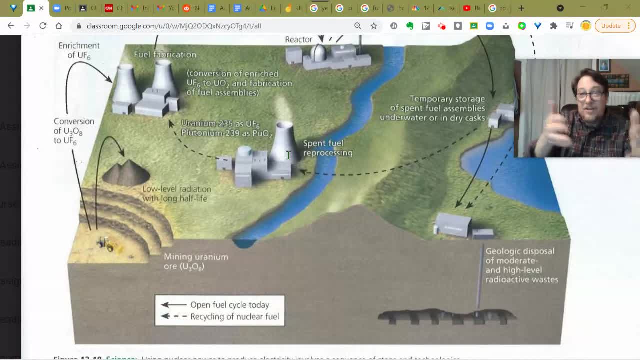 got this coating on it And so reprocessing does the same thing, kind of crushes it all down, puts, gets the stuff you want in the acid, carries it away, reprocesses it. We used to do that here in America. They still do it in other places and we don't do it anymore. It's a very messy process. 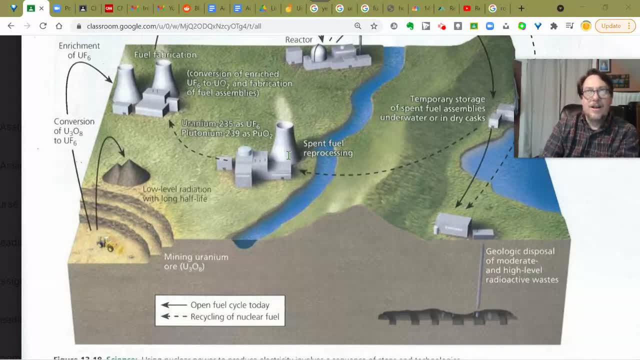 We stopped doing it. in France They even do things like reprocess uranium and plutonium and turn it into glass that is then stored because it can't, like uh, leach out and things like that. But anyway, that's the idea of the nuclear fuel cycle. 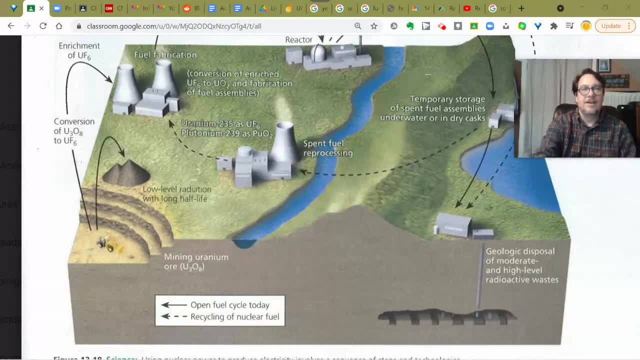 I'm going to say thank you very much for watching this And, uh, I appreciate your time. I'm going to stop now and, uh, I'll see you later. Bye-bye.